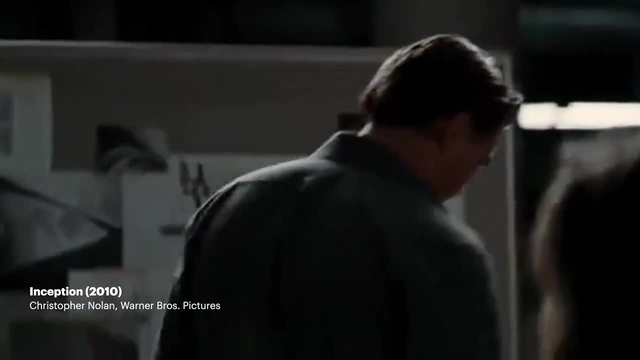 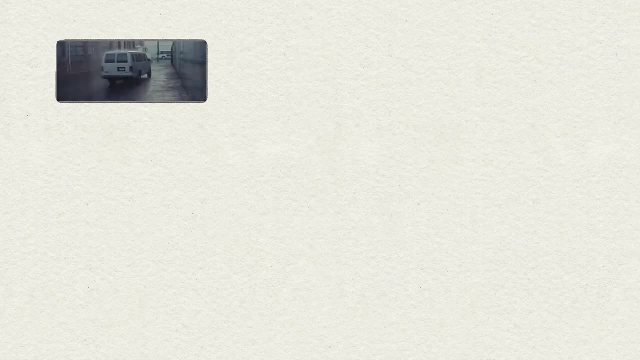 wipe his criminal record clean If he can implant the idea of dissolving a company in the mind of one of his competitors. To be able to implant an idea into someone's subconscious isn't good enough to go into just one dream. He has to go several layers deep. So a dream inside a dream inside a dream. 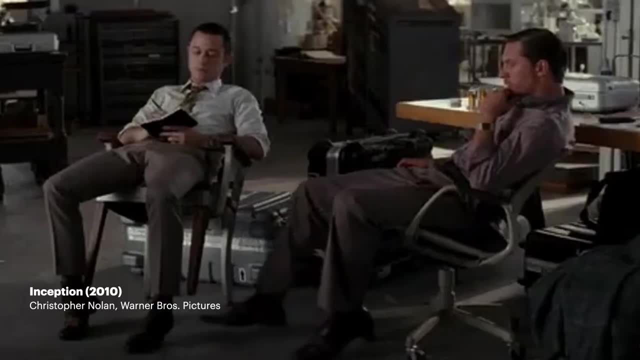 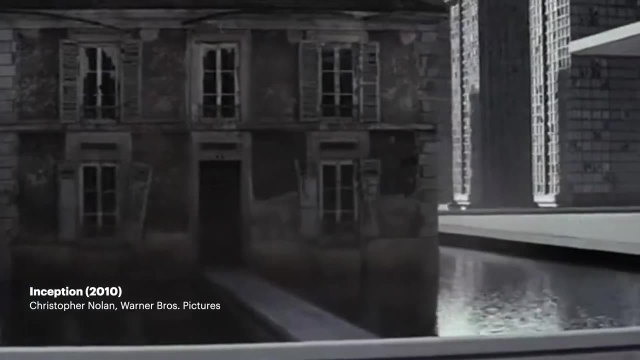 In order to wake someone up from the dream world, they need a kick, a sudden jolt that will wake them up. They also have to be mindful of not going too deep, otherwise they'll enter what they call limbo, A dream realm where anything is possible and you can experience a year in. 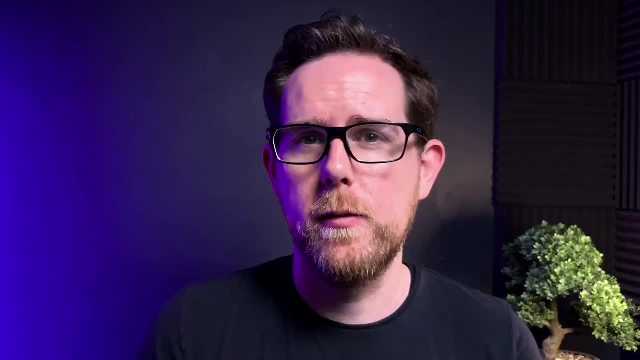 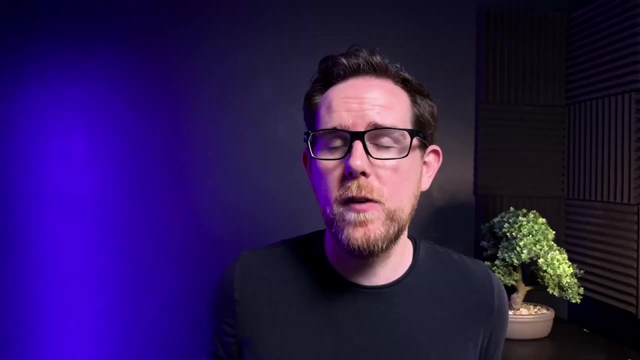 the space of four minutes in the real world. So where am I going with all this? Recursive function is like a dream. It can call itself in the same way that you can enter a dream inside a dream. In your recursive function, you'll always have an exit condition. 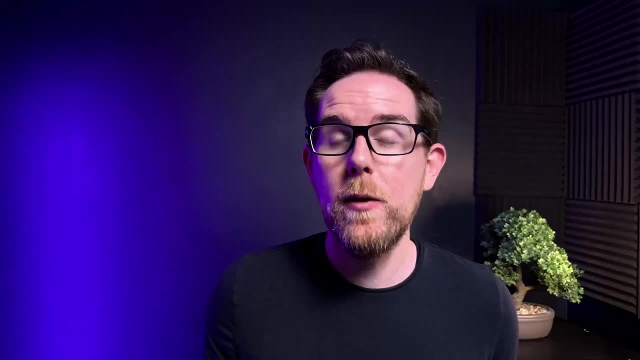 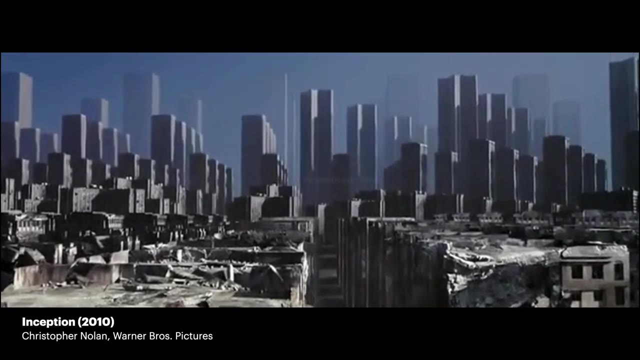 which is like your kick that takes you back up to the calling function. Without this kick- the exit condition- you'll keep going into deeper and deeper levels of recursion and eventually enter limbo, which, in our case, is met with a stack overflow exception. 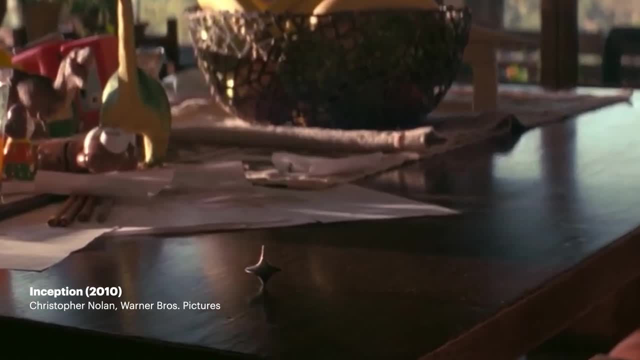 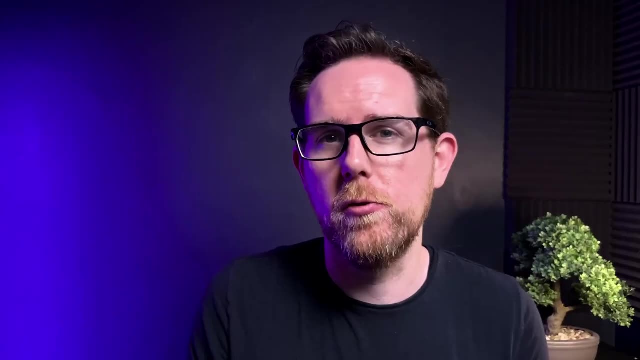 If you still have lots of questions about recursion, like the final scene in Inception, then let's see how we can use it. Recursive functions are mostly used for navigating tree-like structures, like the folder structure on your computer. Each folder can contain other folders. 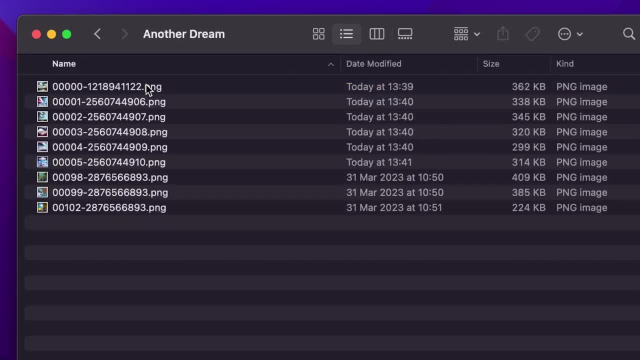 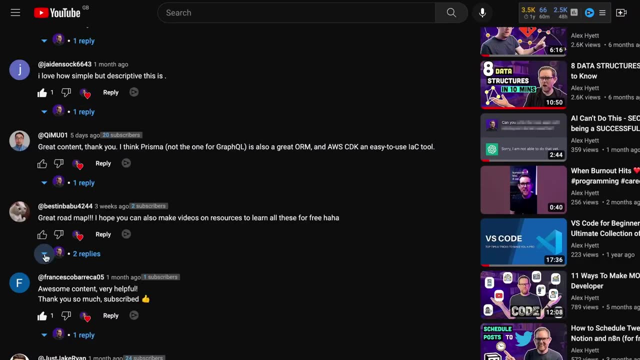 which contain more folders, but eventually you'll get down to a folder that just contains files. Then you have to navigate your way back up the folder structure to get where you started. The same structure can be seen in comment threads on YouTube videos or blog posts. I will be very 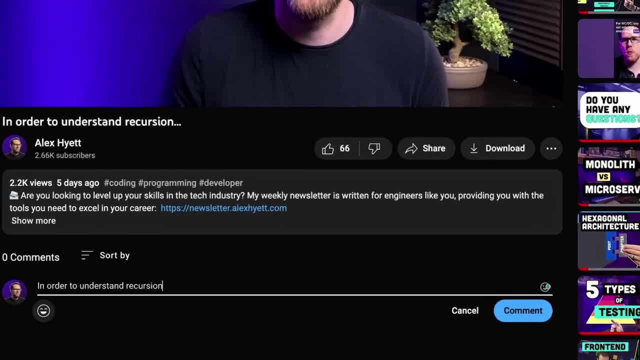 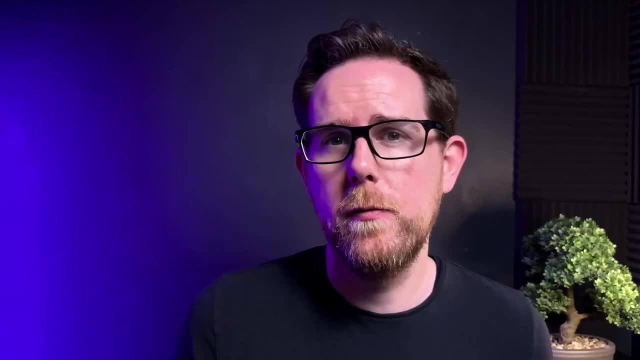 disappointed if no one leaves a recursion thread in the comments, so please leave a comment below. Any place that has an unknown number of nested elements can use recursion to navigate through the file, and you can also use recursive functions to navigate through the file. 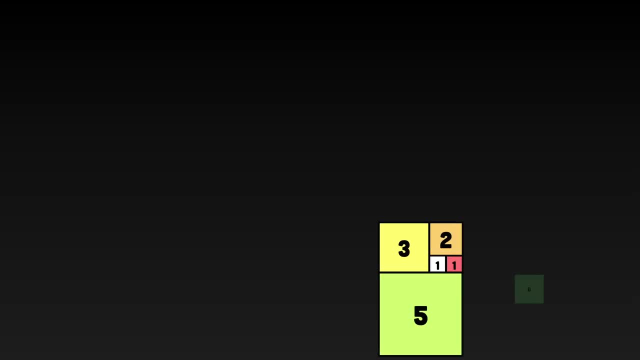 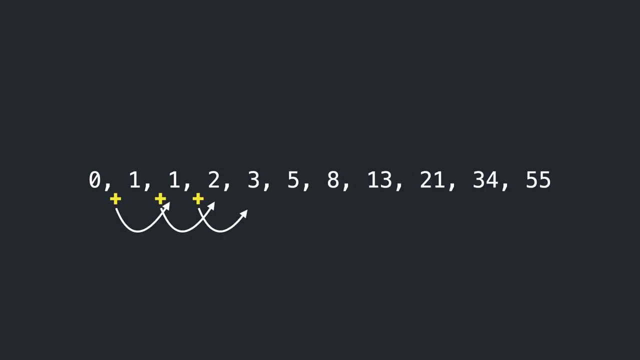 A common example of recursion is calculating the Fibonacci sequence. The sequence starts with 0 and 1, and then the following numbers are calculated by adding up the previous two numbers. So let's say we want to calculate the 10th number in the Fibonacci sequence. 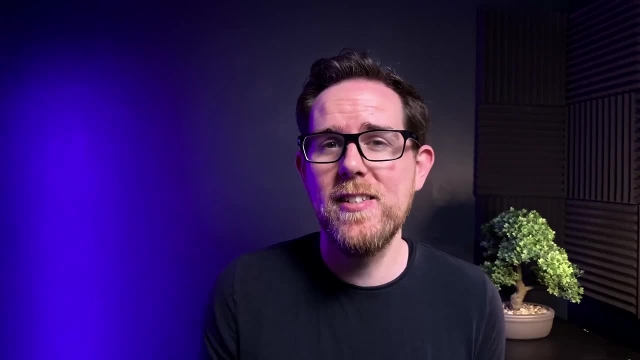 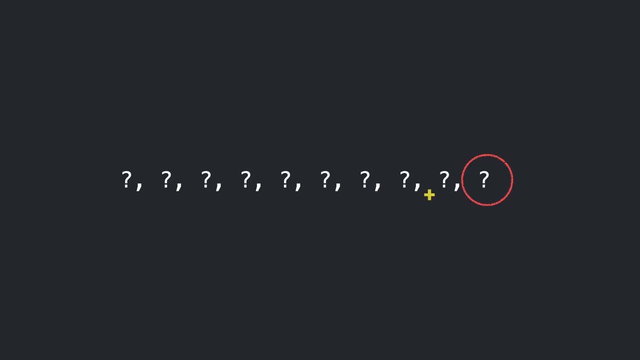 To do that, we can use a recursive function like this one. In this case, n starts from 0, so we need to put in 9 to get the 10th number in the Fibonacci sequence. To work out the 10th number, we need to add up the previous two numbers. We can use this recursive. 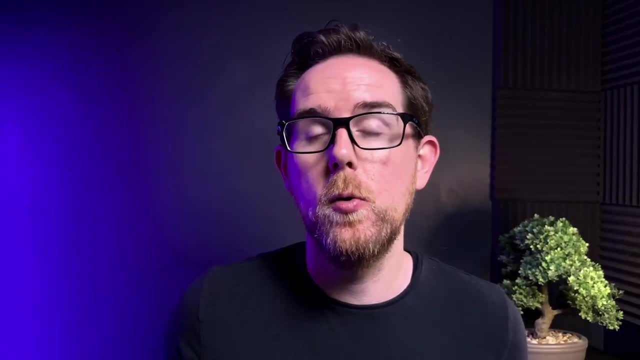 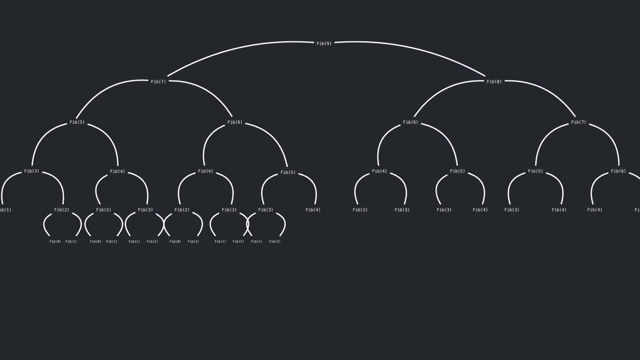 function, to call the recursive function again twice to work them out. But of course we don't know what they are, so we need to call the recursive function again twice in order to work them out. This happens again and again until we get to 0 or 1, where we finally return. 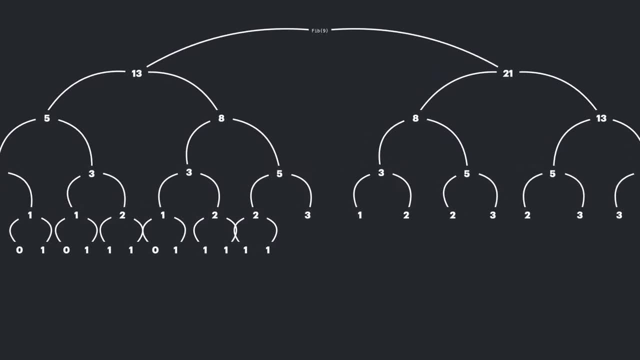 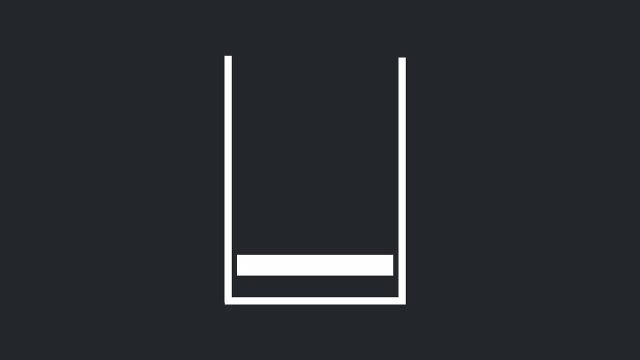 a number and then we work our way back up the call stack to get the final result of 34.. Recursive functions are useful and you get nice simple code, but they're not the most efficient way of doing things. For each call, we have to push and pop methods from the call stack, which often results in poor performance. 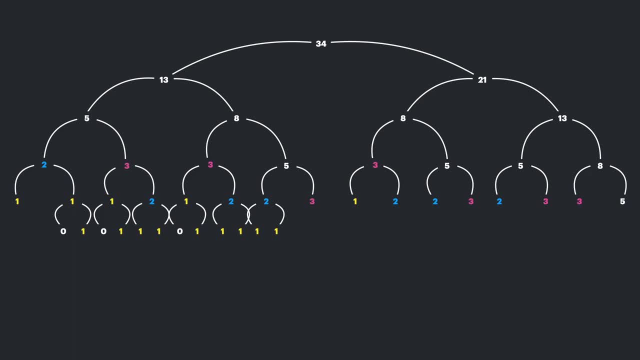 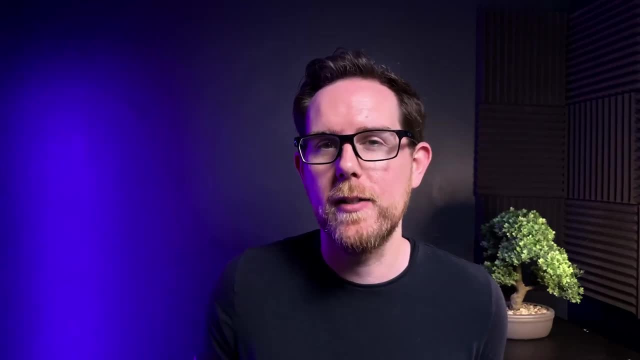 In the Fibonacci code, we also end up calling the function with the same number multiple, multiple times, which isn't very efficient. In this case, you would actually get better performance by doing it in a loop instead of using recursion, especially as we get to. 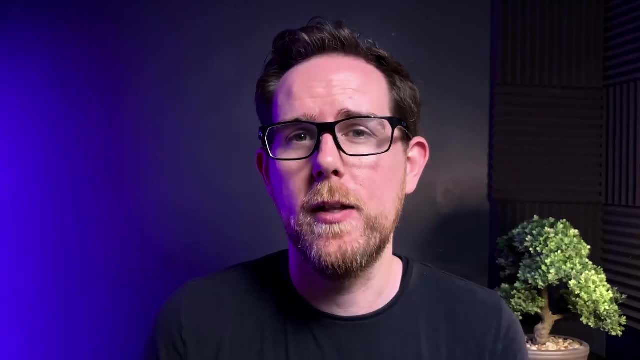 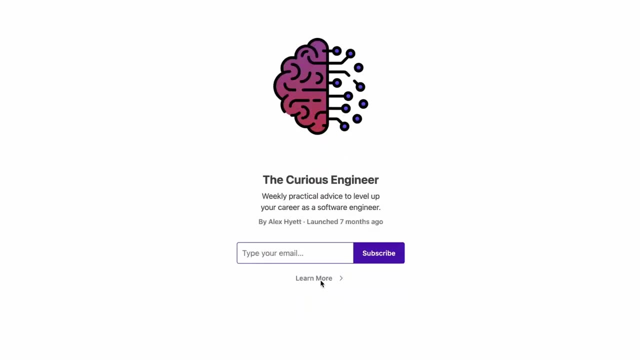 higher numbers. As with all things in programming, it's important that you pick the right tool for the job, and now that you know recursion, that's one more tool that you can use. If you liked this video, then you might also like my newsletter, The Curious Engineer, where I cover topics to help you succeed, as 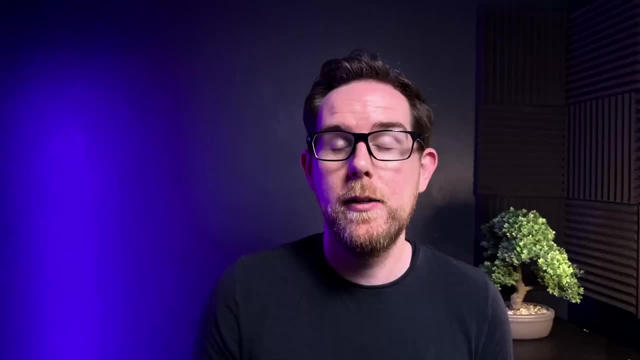 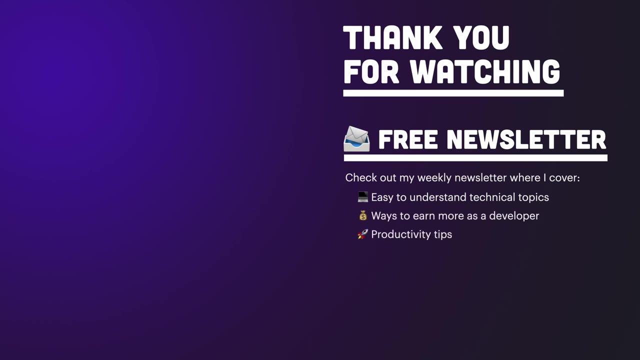 a software developer. There is a link in the description if you want to check it out. Thank you for watching. don't forget to go and watch Inception and I will hopefully see you in the next video. Subtitles by the Amaraorg community. 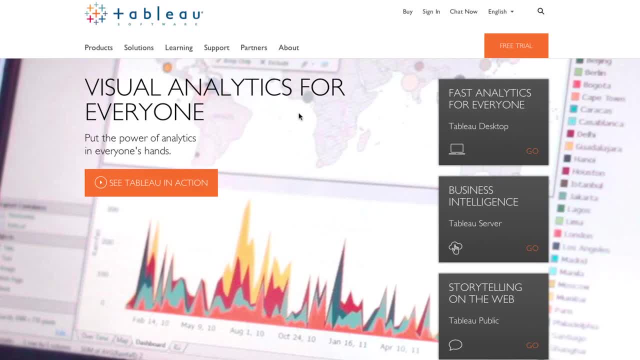 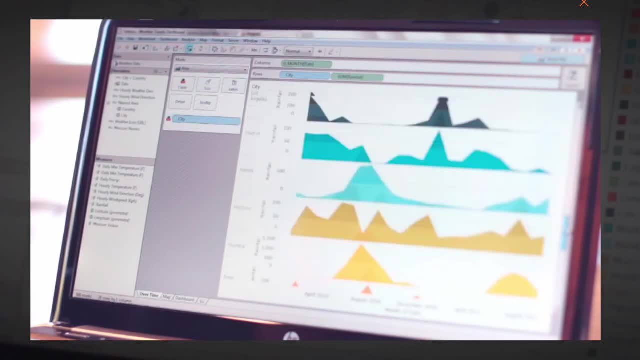 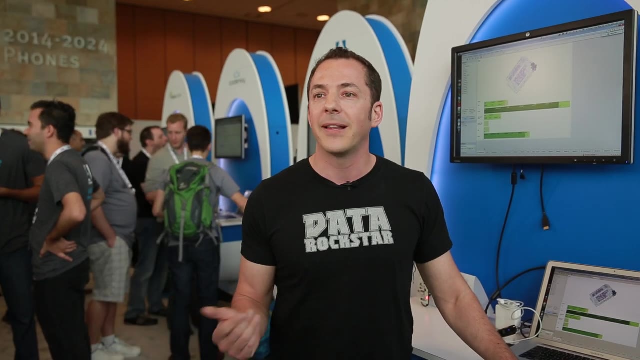 At Tableau. our mission is simple: It's to help people see and understand their data. So the Google Cloud Platform really helps a company like Tableau analyze billions of records of data at internet scale with simple point and click operations- All you need to. 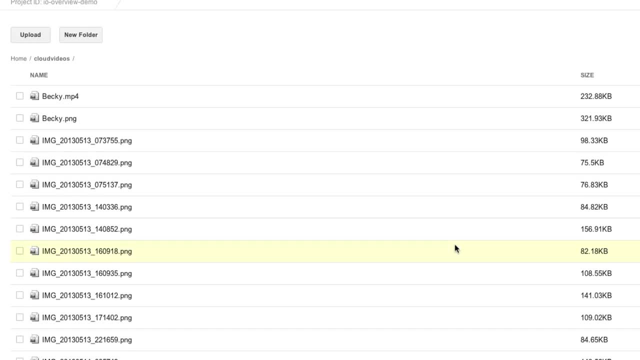 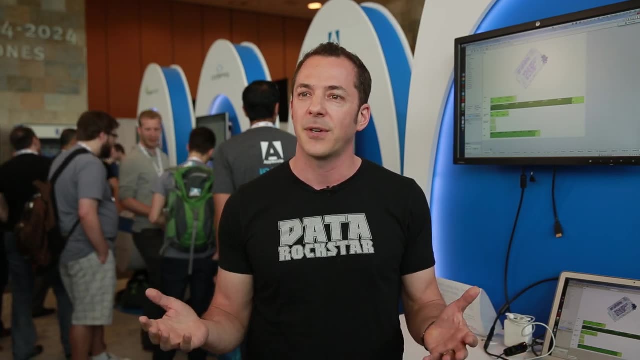 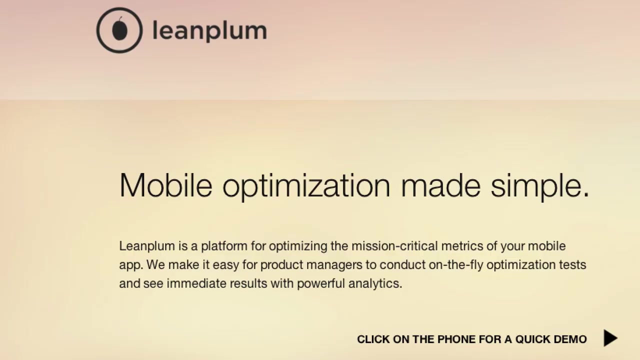 focus on is putting your data in the Google Cloud Platform, and Google takes care of the rest, So you can focus on the core aspects of your business rather than managing all that infrastructure. So we are Lean Plum and we're building a platform to optimize the mission critical metrics of your mobile app. We're a young company, a few less than.